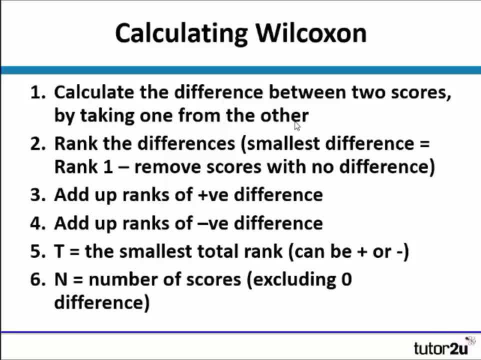 So the first thing that we do is calculate the difference between the two scores by simply taking one from the other. We then rank the differences, add up the ranks of the positive differences and add up the ranks of the negative differences. We find the smallest total rank, which gives us our value of T. 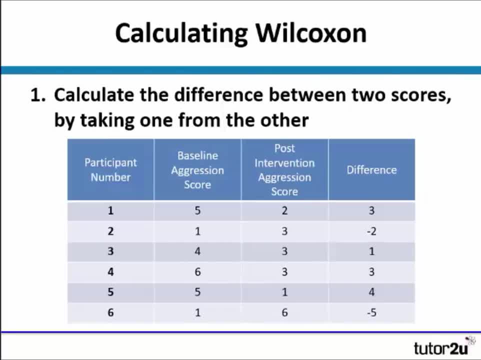 And then we look at the number of scores to help us use the critical values table. So, breaking this down step by step, we need to first of all calculate the difference between the two scores. So 5 minus 2 is 3, 1 minus 3 minus 2, 4 minus 3 is 1, and so on and so forth. 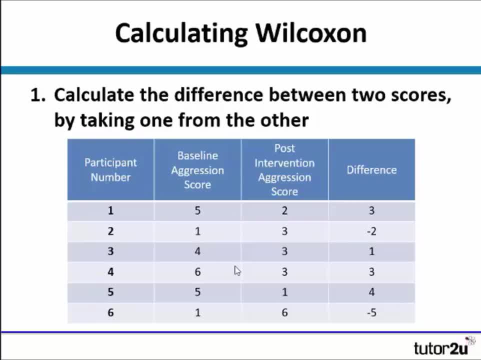 It's really important that you are consistent. Consistent in the way in which you are taking one score from the other, because otherwise it's going to lead to a lot of confusion later on. So these minus numbers are important. The next step is to rank the differences. 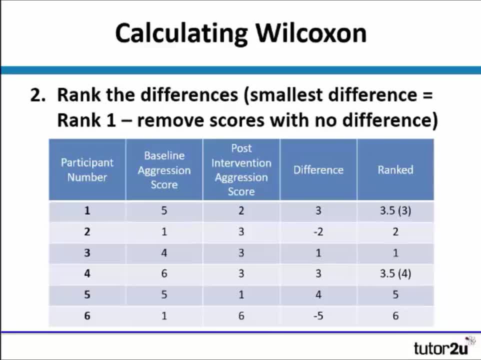 As with all inferential statistics, this is quite an important step. So the first thing we look at is for the smallest number, and that is 1.. So that obviously gets the rank of 1.. Then we have a 2.. It doesn't matter that it's a minus number for now, but it gets the rank of 2.. 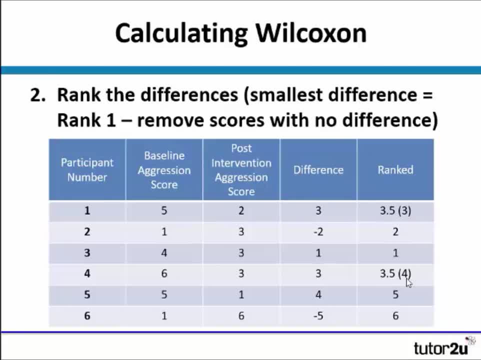 We then have two 3s, So they would get A rank of 3 and 4.. Obviously, we can't do that, so we have to give them an equal ranking, which is 3.5.. And then we have 5 and 6.. 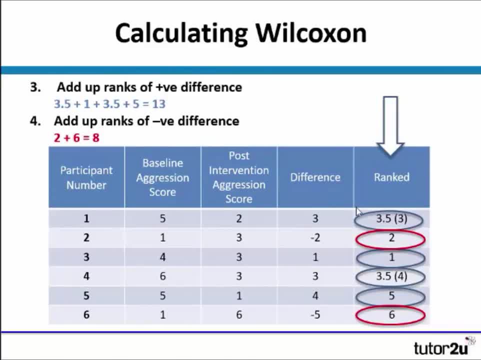 The next thing that we do is add up the ranks of the positive difference, which I've circled in blue, So we have 3.5, 1,, 3.5 and 5,, which adds up to 13.. And then we add up the ranks of the negative differences, which is 2 and 6,, which is 8.. 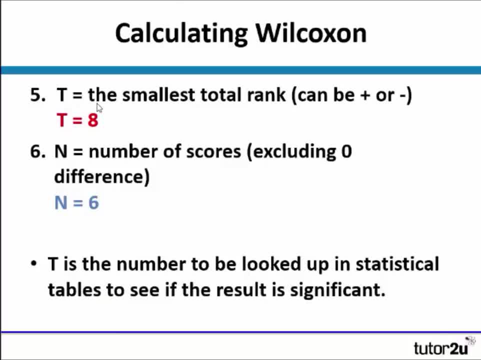 The information that we use to use the critical values table is t, which is the smallest of the total ranks. So it doesn't matter. It doesn't matter which one we're using, as long as it's the smallest one, And our smallest rank was t equals 8.. 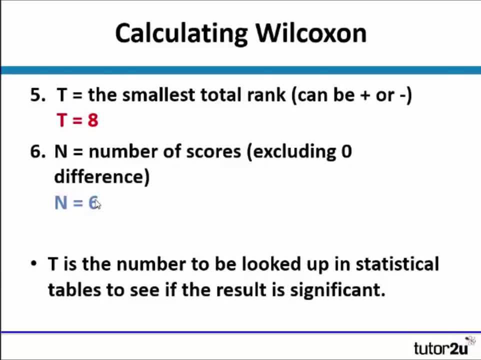 We then use the number of scores excluding any that had no difference. In this example, we didn't have any scores of no difference, So that's fine. So these are two pieces of information we need to use to look up in the statistical tables to see if our result is significant. 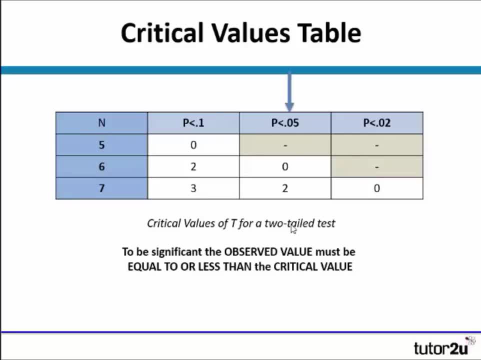 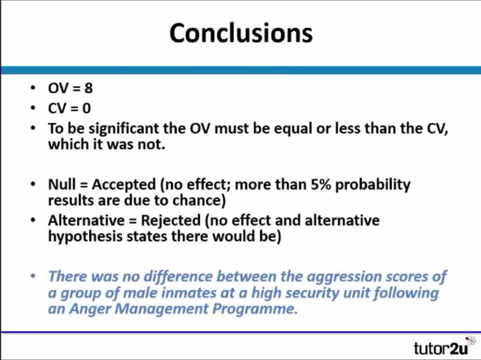 So we're going to be looking at a two-tailed test, And to be significant, our observed value must be equal or less than the critical value, And so we had six participants, So our score needs to be less than zero. Unfortunately, eight is not.